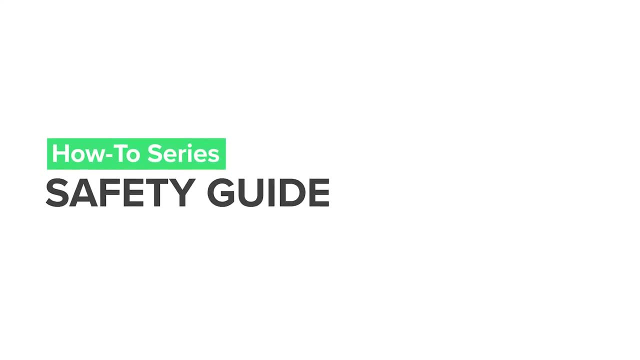 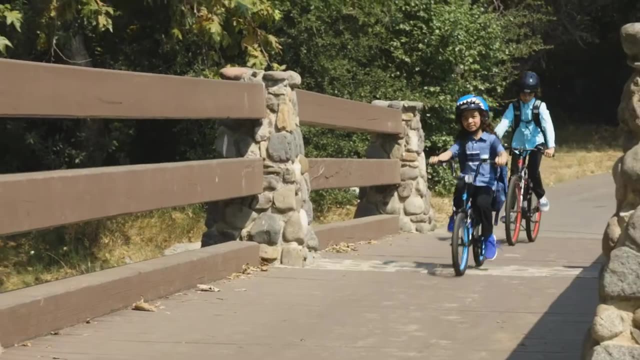 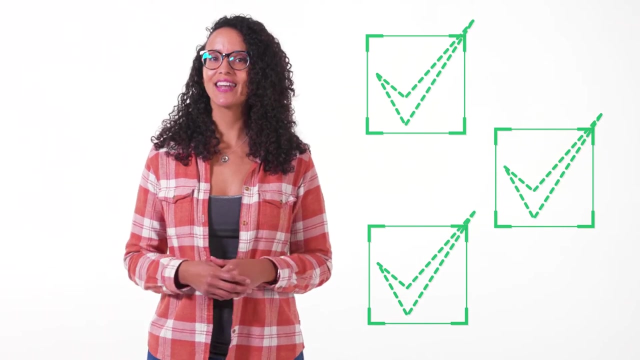 Safety is one of the most important parts of riding a bike. While riding on a great adventure or speeding through the park and trails, you need to have all those safety boxes checked to ensure your child has the safest biking experience possible. Today, let's review some. 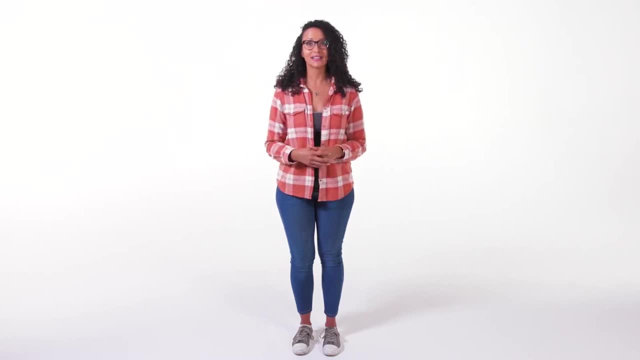 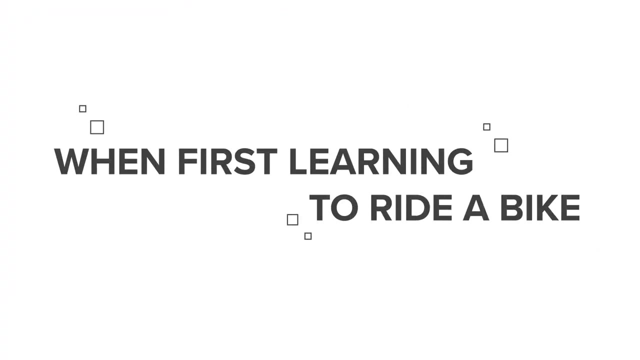 fundamentals of bike safety, protective gear and bike maintenance. to keep your child safely riding, Let's start with the proper protective equipment When first learning to ride a bike. we recommend a helmet. good closed-toed shoes—never let your kids ride barefoot or in sandals—and 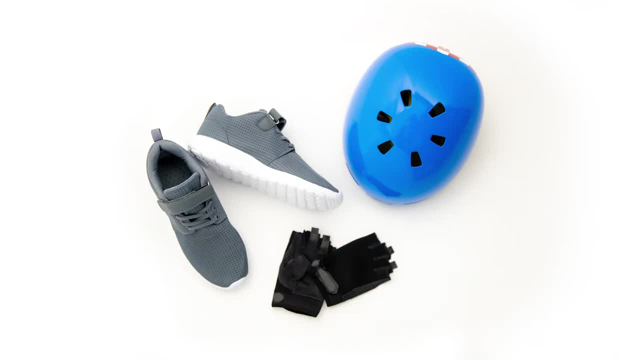 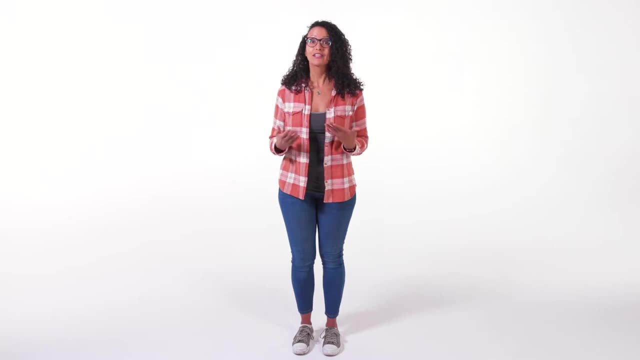 gloves Just in case they fall. it will protect their hands while also improving handlebar grip. Now the helmet is a very important element when riding a bike. It's essential to have a properly fitted helmet for your child. For the right fit, make sure the helmet sits, no more. 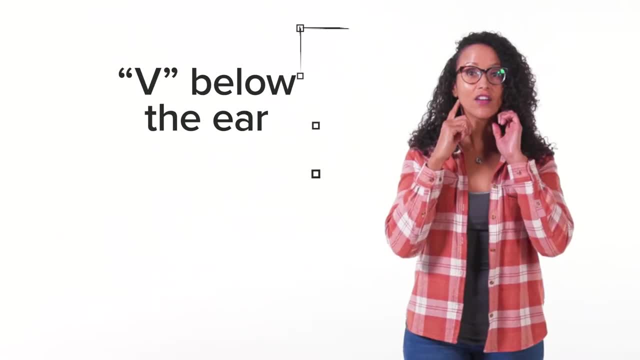 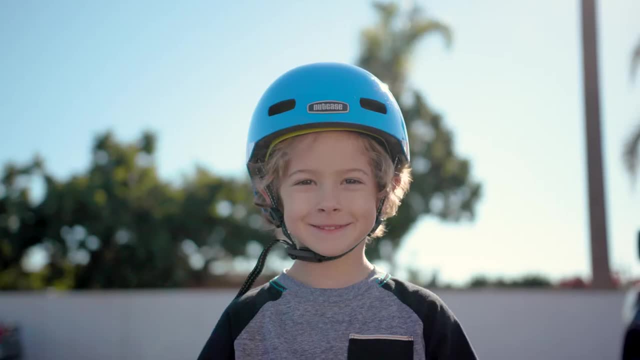 than two fingers above your kid's eyes. Check that the V on the side straps hang below their ear and you can fit no more than two fingers between their chin and the strap While riding. teach your child not to push the helmet back It. 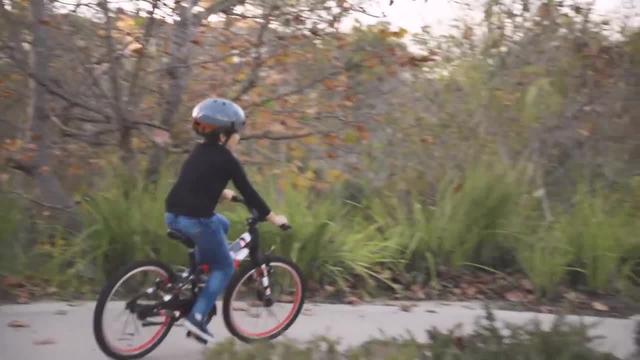 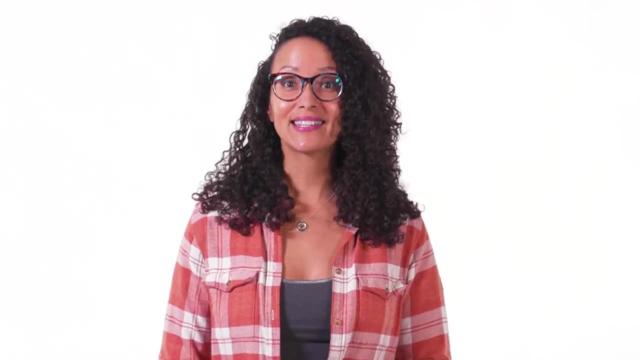 should cover their forehead for proper protection, Keep it fastened at all times When removing and storing, remind your child not to drop the helmet on the ground. Let's take a look at some bike safety factors. Once your child gets moving, it's important. 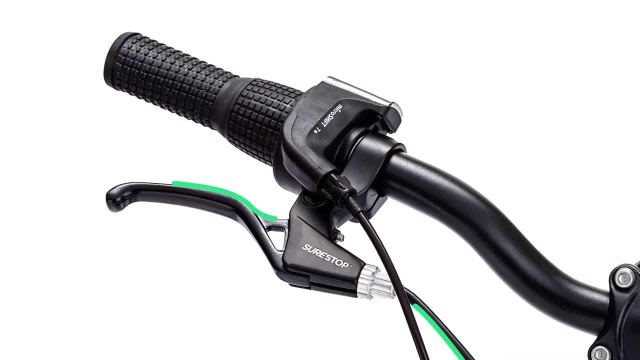 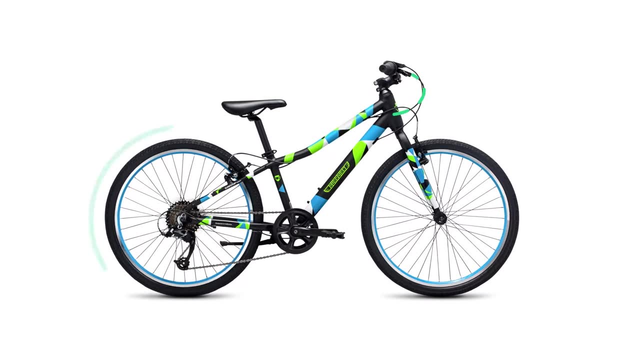 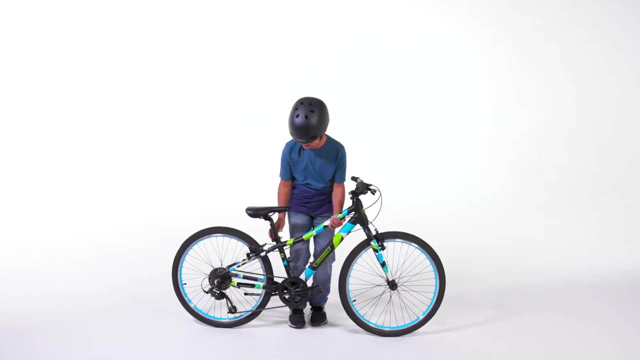 for them to be able to stop safely. All our bikes have our kid-friendly SureStop braking system. This system provides kids with only one brake lever to squeeze, which distributes braking power to both wheels for a faster, safer stop, while also preventing over-the-handlebar accidents. 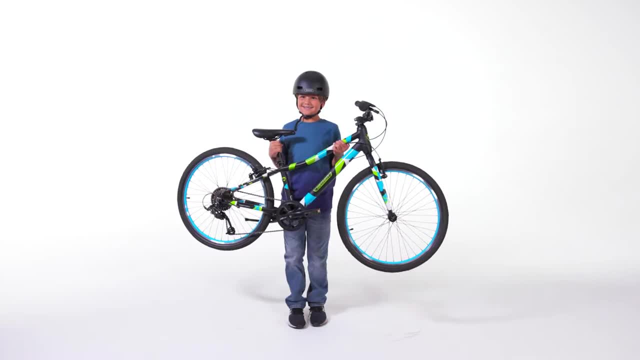 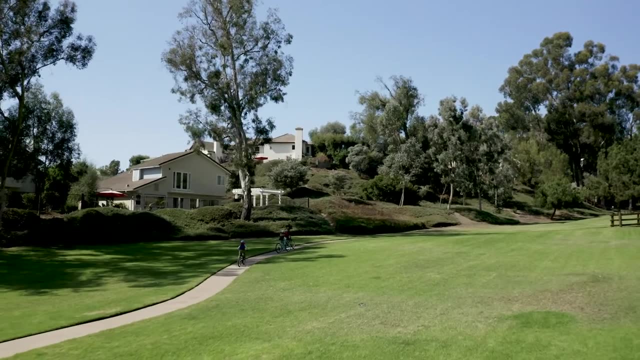 Your child's bike should be less than half of your child's weight. If the bike is heavy and clunky, which most mass-market bikes are, they become difficult to control for a young rider. Here at Guardian Bikes, we want to keep that experience as positive and as safe. 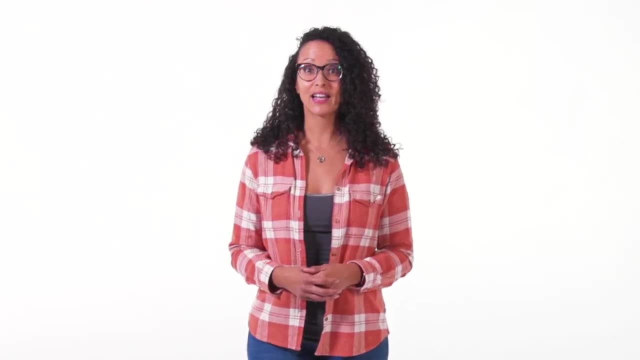 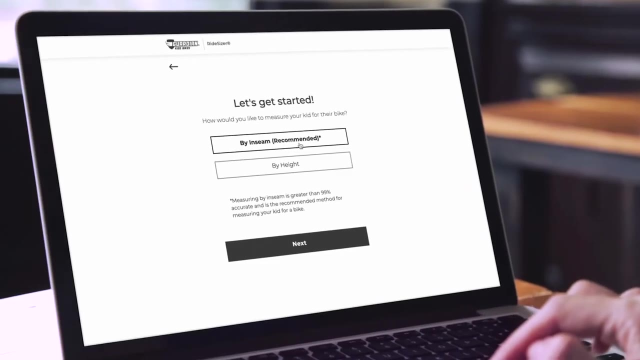 as possible. Size is an important factor when riding a bike. When size is important, it's not just about the size: When sized incorrectly, it can make riding cumbersome and even dangerous for your child. Online at GuardianBikescom, we've created a simple bike sizing tool to 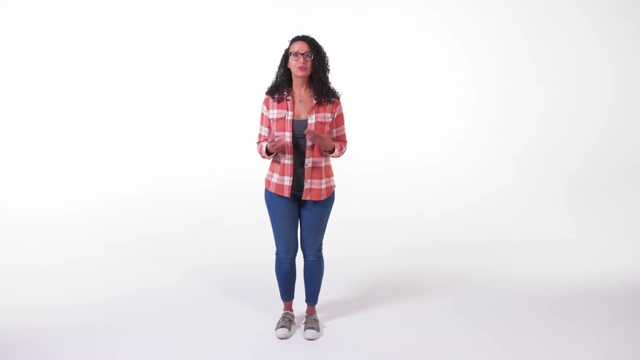 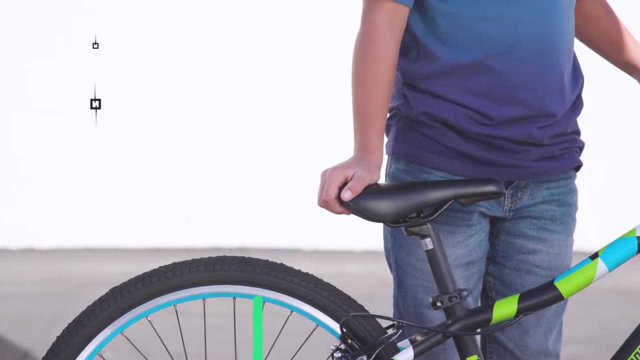 help select the perfect size bike for your child. With the right bike size for your child selected, you'll want to adjust the seat height to fit as well. Minimum seat height should be at most two to three inches above your child's inseam If they are just starting. 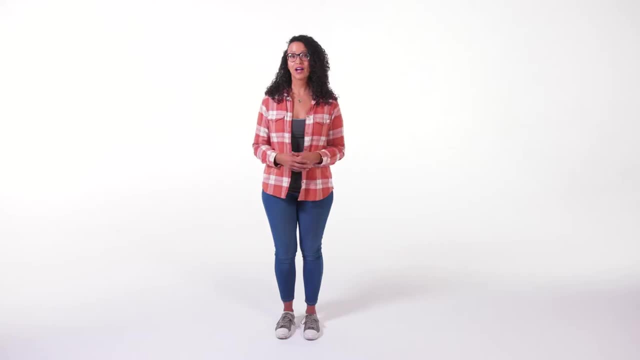 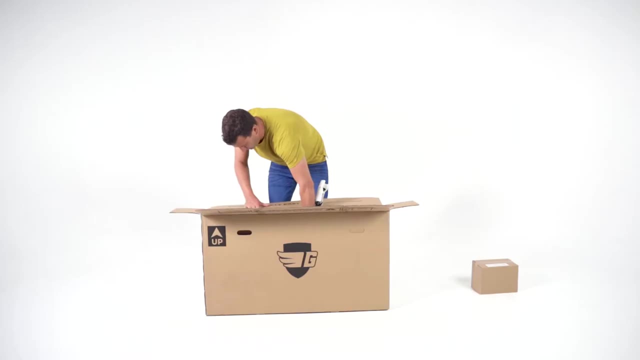 out, line the seat up with their inseam. In order to safely ride your new bike, it needs to be assembled properly. Other cheap bikes typically arrive with boxes of parts and unclear directions. Guardian Bikes come almost fully assembled and ready to go in ten minutes. or less After assembly. it's important to maintain the bike to ensure ongoing safety. A child's bike is meant to be ridden through all the adventures they can find. To keep the adventures coming, it's a good idea to get in the habit of checking in on the bike. 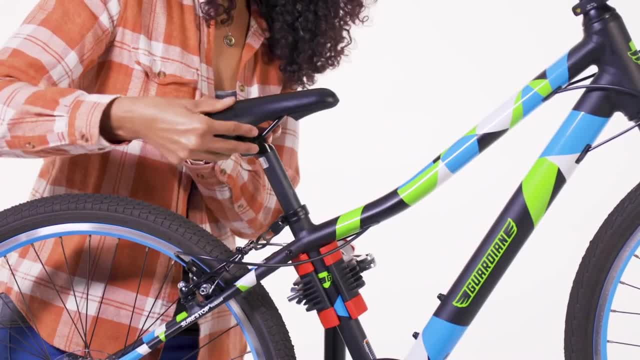 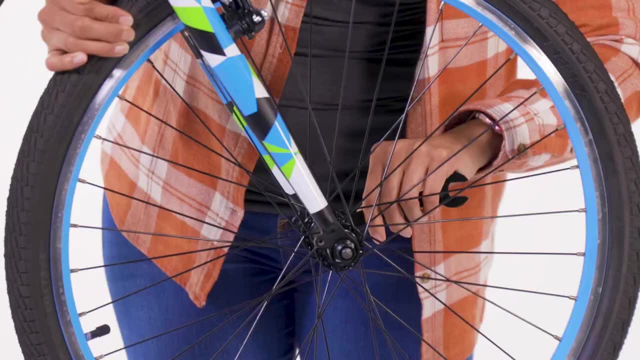 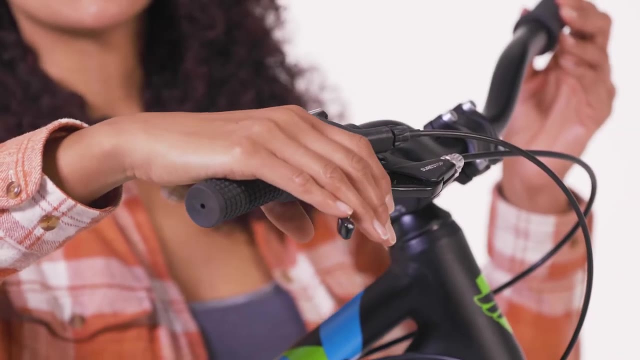 every so often, Let's start by checking that the seat is tight and still sized correctly. Then double check that the handlebars and wheels are firmly attached. While checking the wheels, check the brakes to make sure they're not sticking. Grab the lever and squeeze. 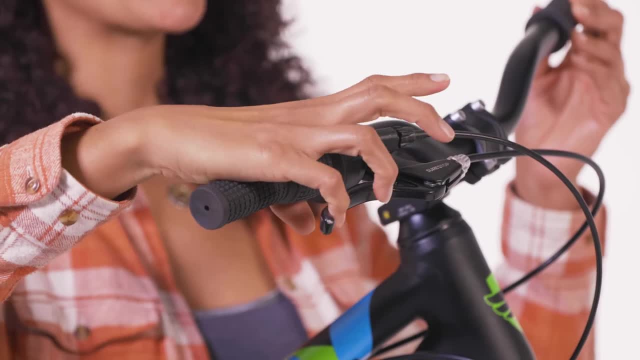 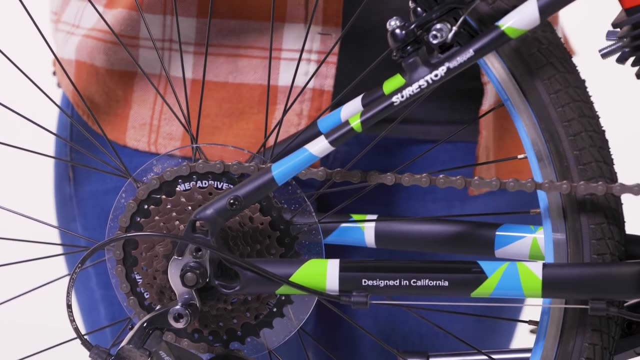 You should be able to fully squeeze the brake with your pinky finger Once a year. we recommend oiling the bike chain. If you notice it's noisy, sticky or see rust, go ahead and oil it. Lastly, give the tires a good squeeze to ensure they are firm. If you notice any. 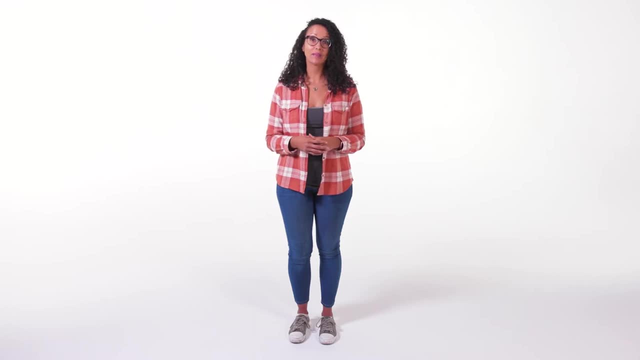 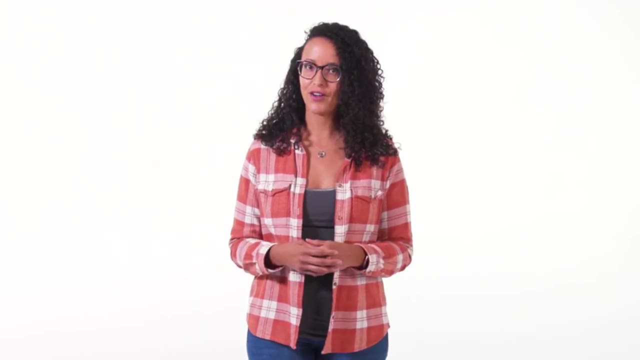 rust. you may need to air them up occasionally. Check the side of the tire for the recommended air pressure. When riding a bike, safety should always be number one. There are basic road rules that every rider should follow, even a supervising adult, When approaching a crosswalk. 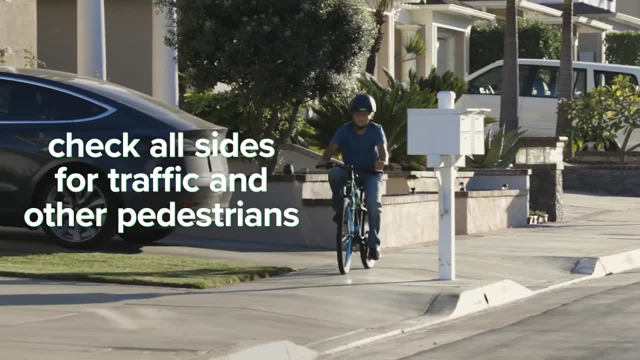 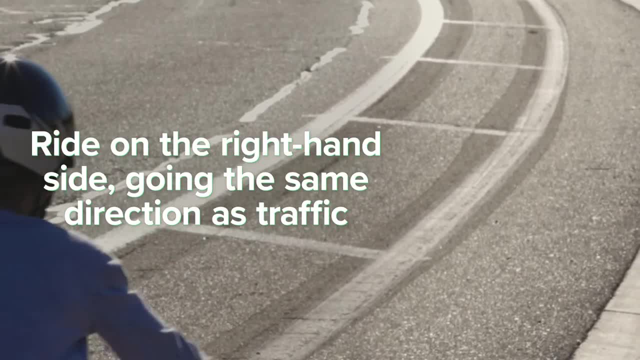 driveway or tight space. check all sides for traffic and other pedestrians. If on the road, try to stick to roads with bike lanes. when possible, Ride on the right hand side of any road trail or sidewalk. you're on going the same direction as traffic. 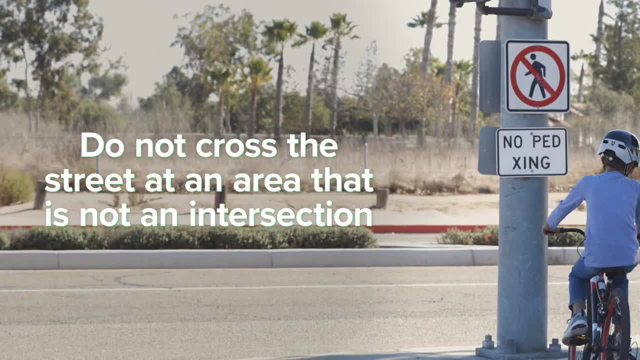 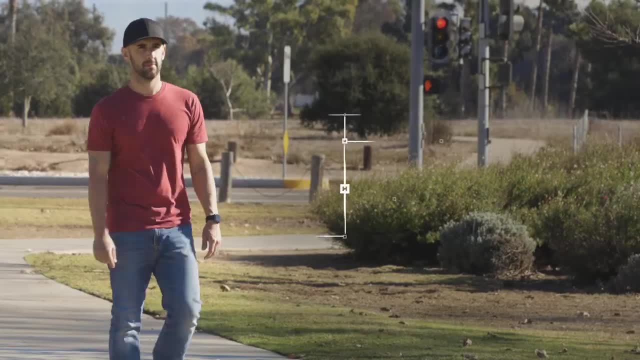 Do not cross the street at an area that is not an intersection. Pay close attention to stop signs and red lights. You're expected to follow the same rules as drivers When passing a biker or a pedestrian. pass them on their left while calling out on your left. 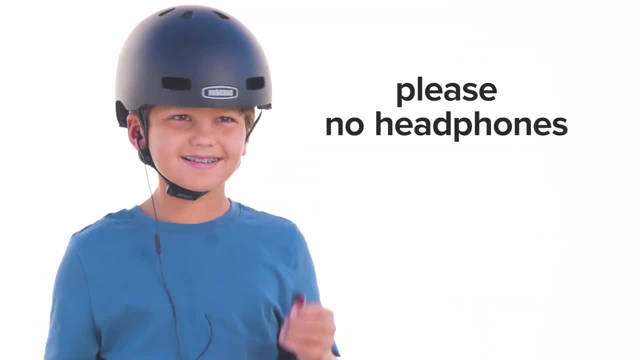 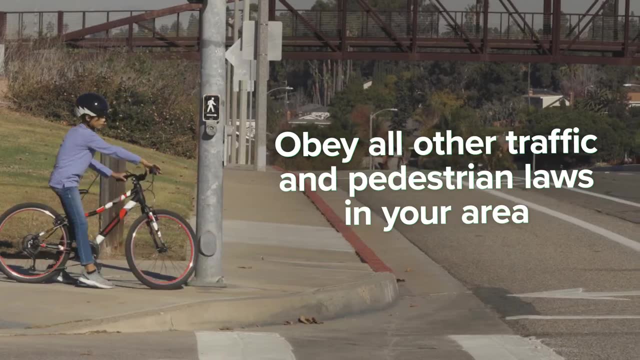 as you approach, You'll want to hear noises from cars, pedestrians and other bikes, so please, no headphones. Obey all other traffic and pedestrian laws in your area. Now that we've covered basic safety, I want you to understand how to make sure your bike is in.